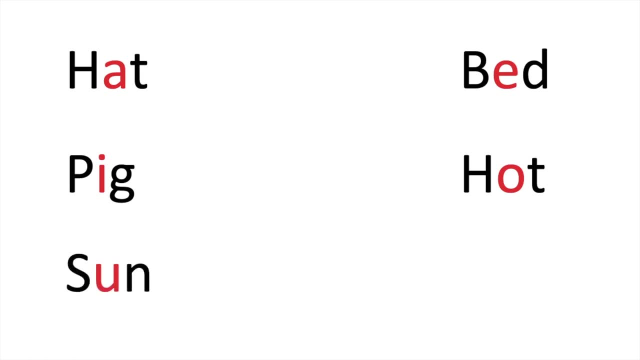 Sun, Sun. S is a consonant. U is a vowel. N is a consonant. U is a vowel. N is a consonant. is a vowel. N is a consonant Road. The letter R is a consonant. O and A are both vowels. 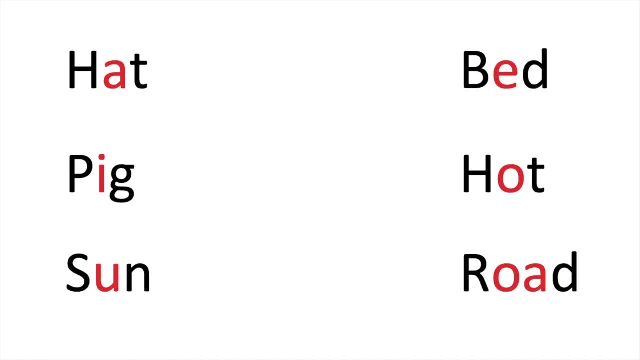 and the letter D is a consonant. Now let's see how the letter Y can act as a vowel and a consonant. Let's start with vowel, For example sky. Here the letter Y makes an I sound. The letter I is a vowel. Therefore, in this example, the letter Y is considered to be a vowel. 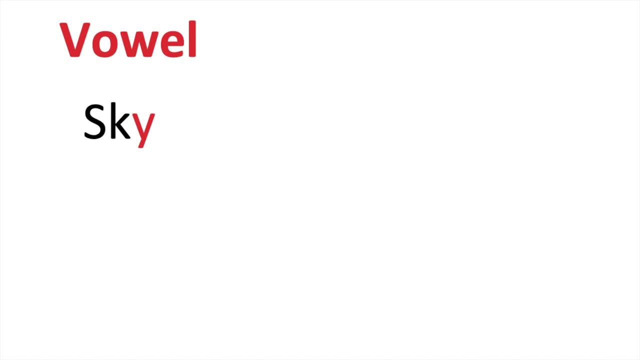 It's important to remember that the letter Y is a vowel when there are no other vowels in the word. So, as we can see here, the letter S is a consonant, the letter K is a consonant and the letter Y is a vowel. There are no other vowels in the word. 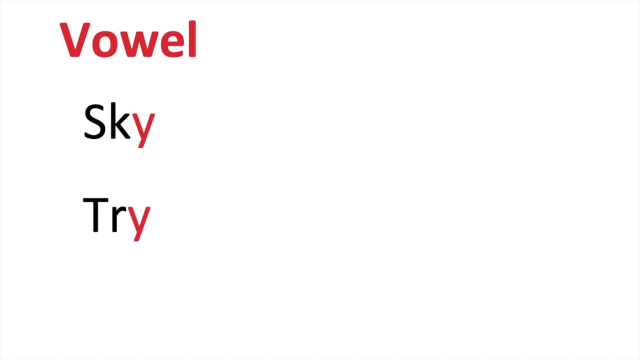 Another example is: try Again. the letter Y makes an I sound, Therefore it's considered to be a vowel. Angry. Here the letter Y makes an I sound, Therefore it's considered to be a vowel. The letter E is a vowel, Therefore, in this example, the letter Y is considered to be. 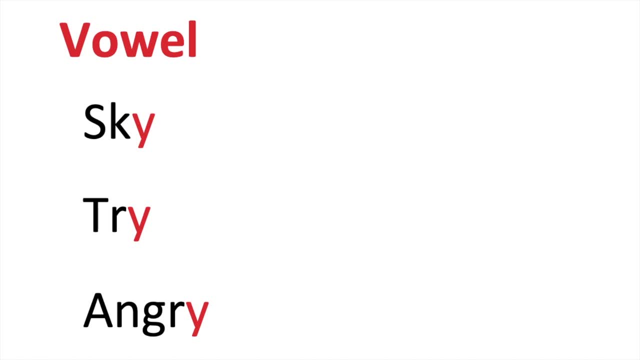 a vowel, The letter Y is considered to be a consonant when it comes at the beginning of the word and makes the Y sound, For example, yellow, You, You, Yelp. Each vowel has a short and a long sound. Vowel A Short sound is a Apple Cat. The long sound is a Cake Bake. 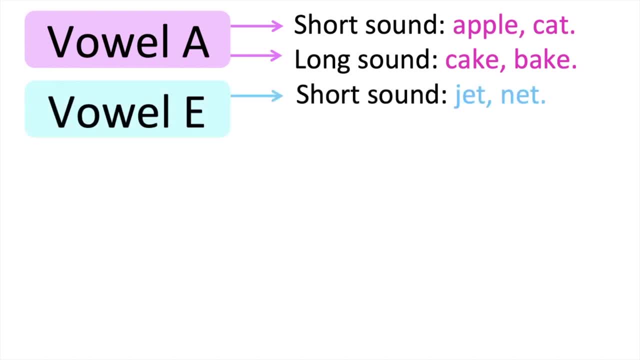 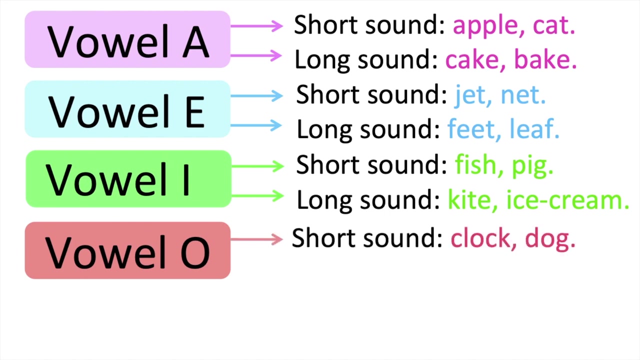 To To, To do, Todo, Todo, Todo, Todo. Feet Leaf. Vowel I. The short sound is I Fish outbreak Pig. The long sound is I Qit ice cream. Vowel O, The short sound is O Clock Dog. The long sound is O Rope Boat. 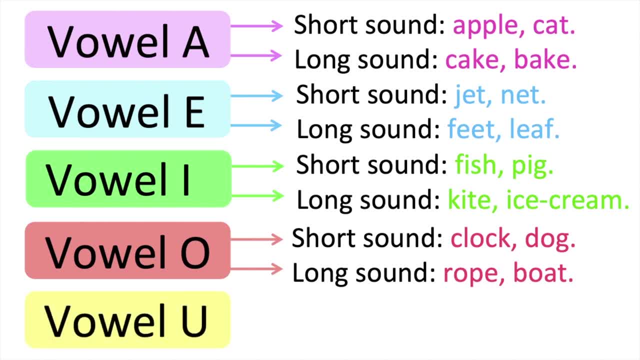 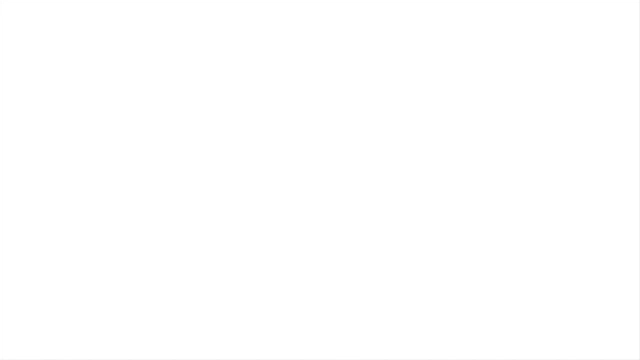 Vowel U. The short sound is A Sun Jump. The long sound is U Cute Unicorn. There are two rules you can follow which will make reading words easier. The first is when you have one vowel in a word. Here the vowel sounds like its short sound. For example jam, The vowel is A. 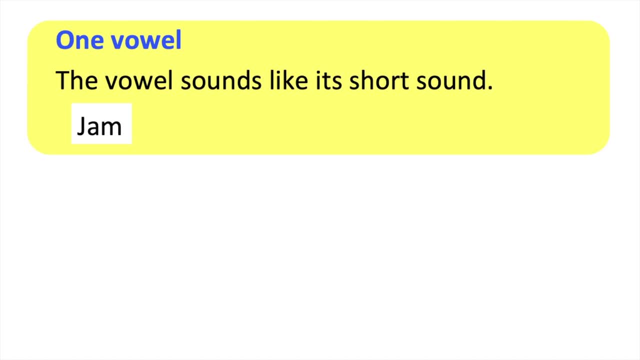 It makes the short sound A Jam Bed Had. If there are two vowels in a word, then the first vowel sounds like its alphabet name and the second vowel is silent. For example, bake. Here there are two vowels, A and E. The letter A makes its. 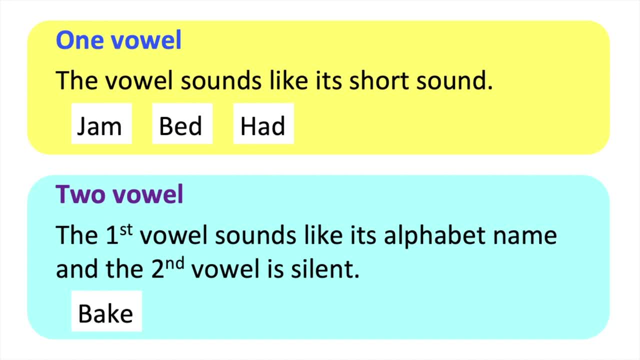 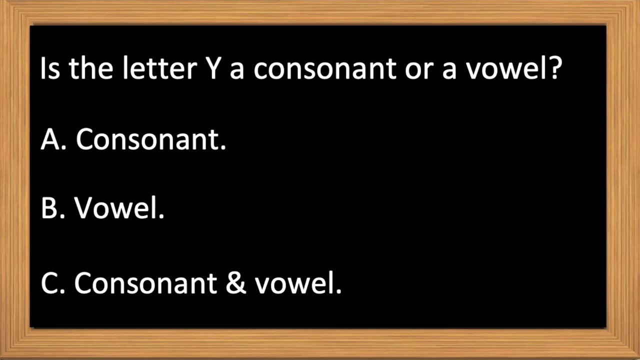 alphabet name, which is the long sound A and the letter E is silent. Bake, Same Coat. Again, here we have two vowels. However, I only pronounced the first vowel, sound Coat. I know, sometimes I make the count of the twice of the first vowel, but I